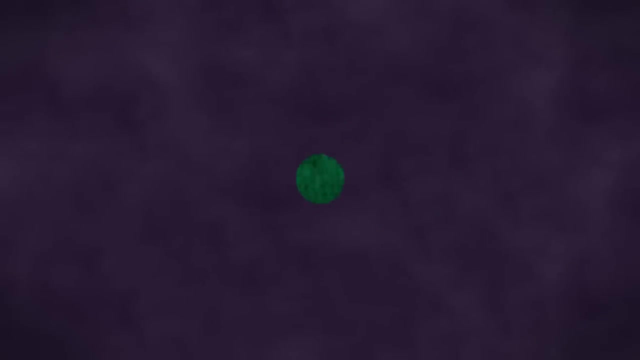 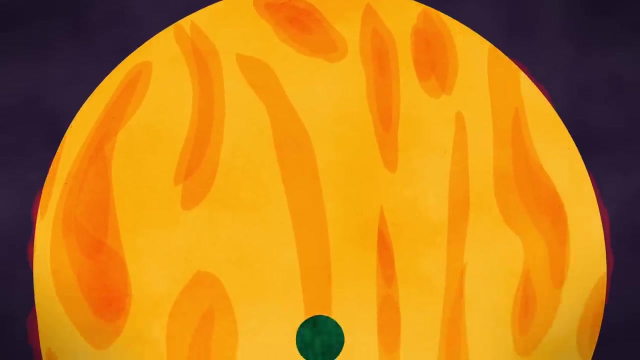 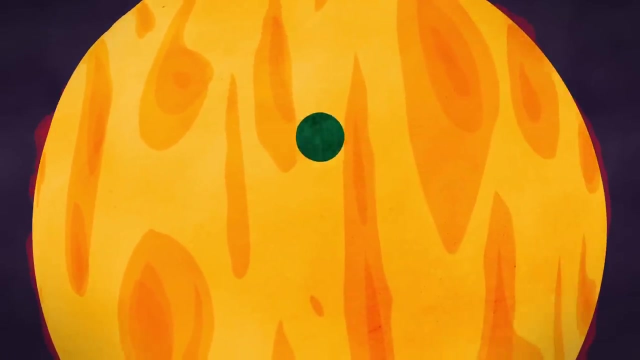 But the original star's angular momentum is preserved. So for the same reason that a figure skater's spin accelerates when they bring in their arms, the neutron star spins much more rapidly than its parent. The fastest neutron star on record rotates over 700 times every second. 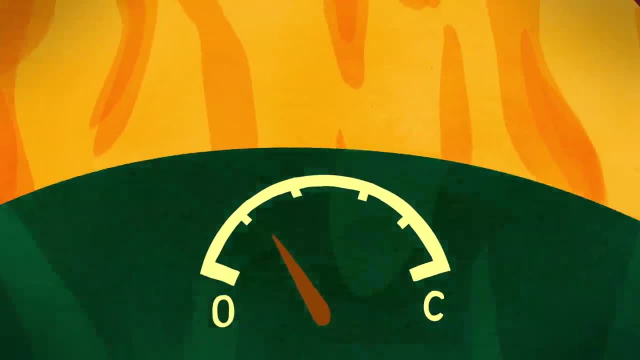 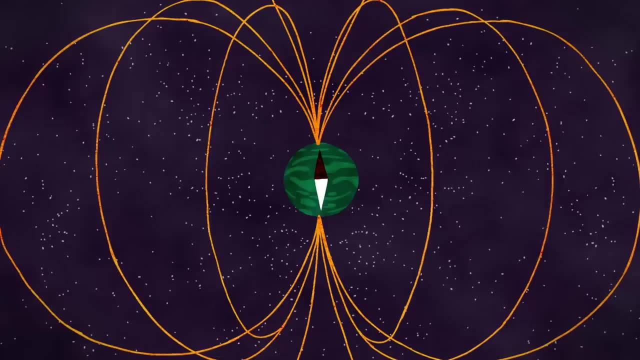 which means that a point on its surface whirls through space at more than a fifth of the speed of light. Neutron stars also have the strongest magnetic field of any known object. This magnetic concentration forms vortexes that radiate beams from the magnetic poles. 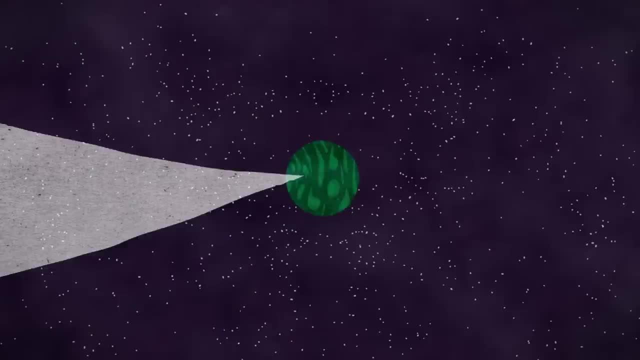 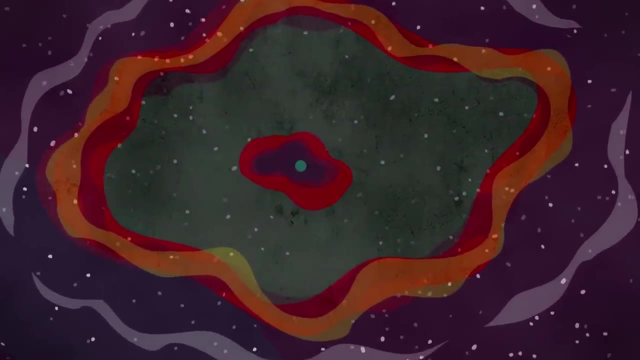 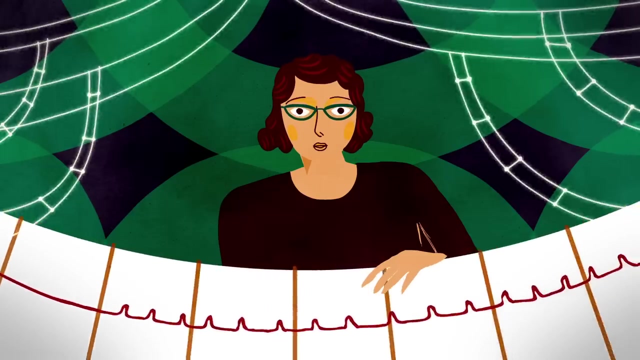 Since the poles aren't always aligned with the rotational axis of the star, the beams spin like lighthouse beacons which appear to blink when viewed from Earth. We call those pulsars. The detection of one of these tantalizing flashing signals by astrophysicist Jocelyn Bell in 1967. 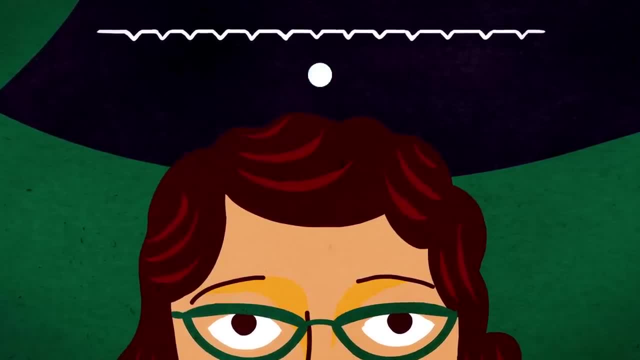 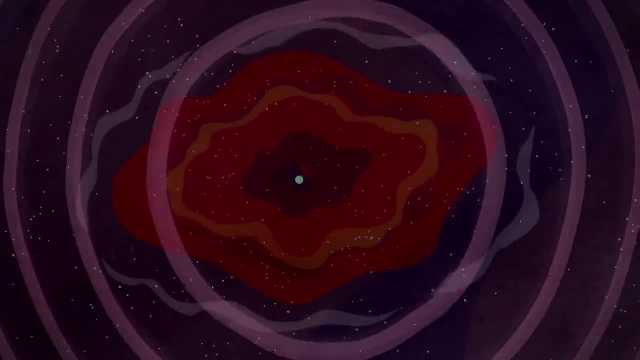 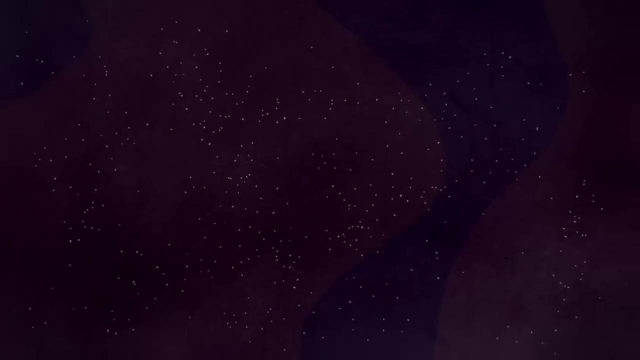 was in fact the way we indirectly discovered neutron stars in the first place. An aging neutron star's furious rotation slows over a period of billions of years as it radiates away its energy in the form of electromagnetic and gravity waves. But not all neutron stars disappear so quietly. 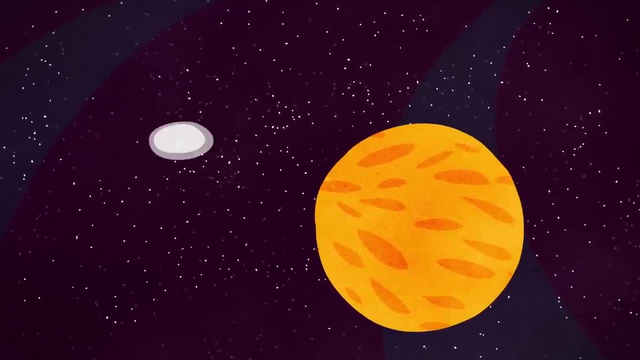 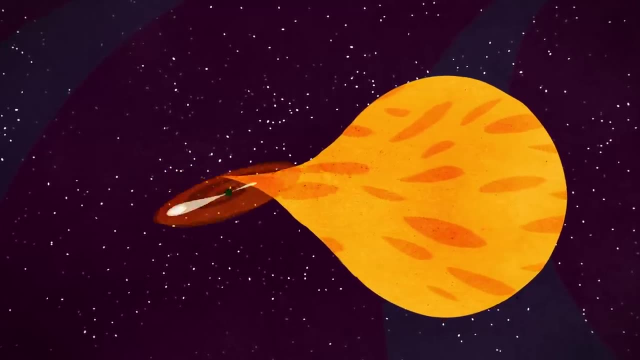 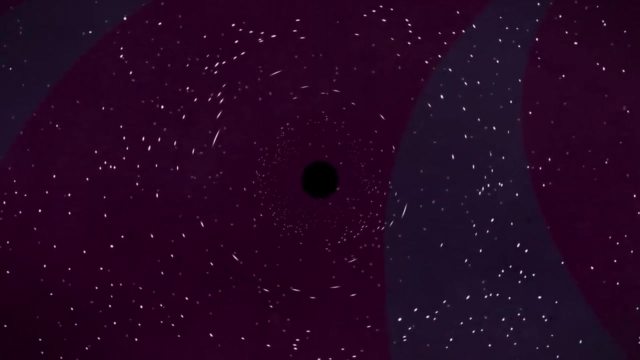 For example, we've observed binary systems where a neutron star co-orbits another star. A neutron star can feed on a lighter companion, gorging on its more loosely bound atmosphere, before eventually collapsing cataclysmically into a black hole. While many stars exist as binary systems, 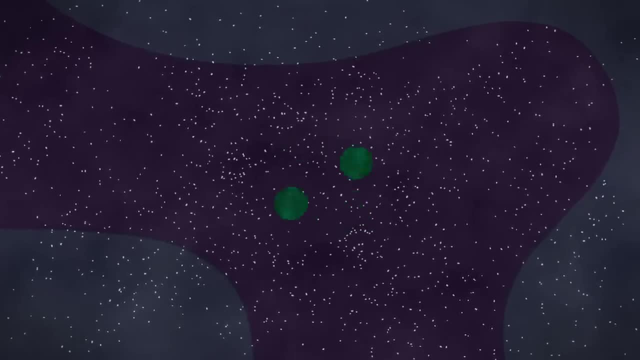 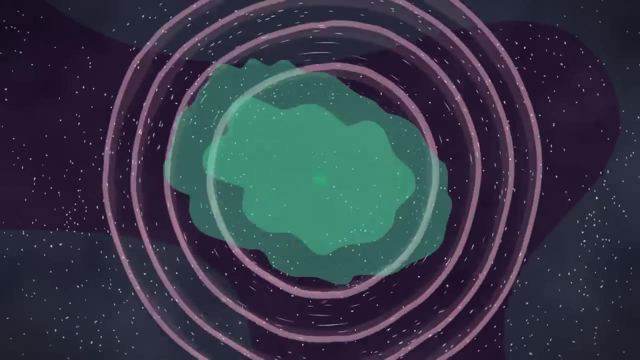 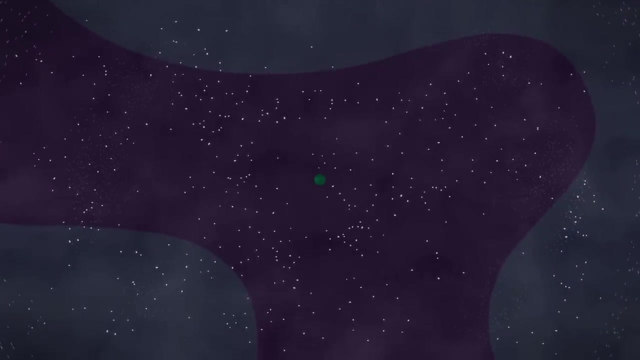 only a small percentage of those end up as neutron star binaries, where two neutron stars circle each other in a waltz doomed to end as a merger. When they finally collide, they send gravity waves. gravity waves through spacetime like ripples from a stone thrown into a calm lake. 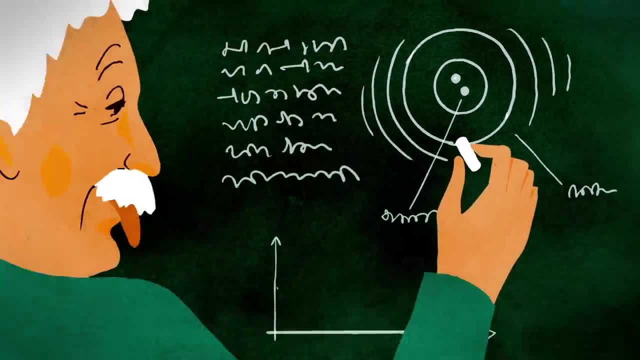 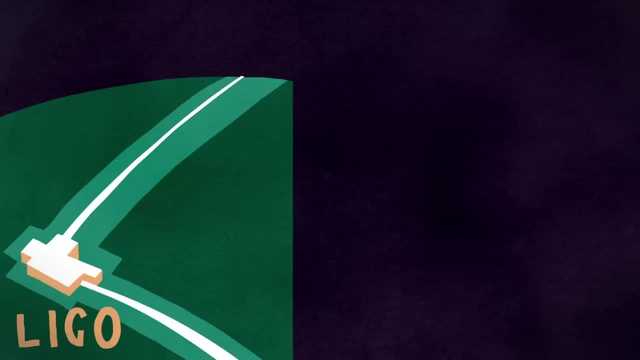 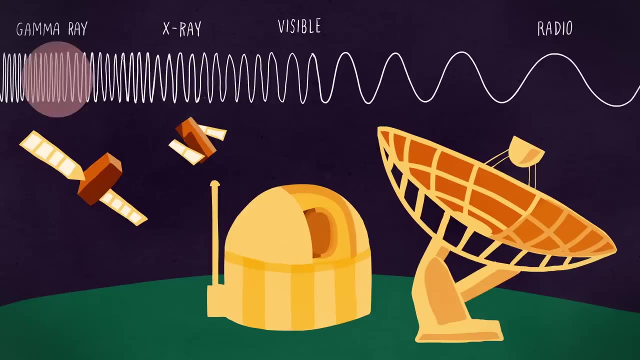 Einstein's theory of general relativity predicted this phenomenon over 100 years ago, but it wasn't directly verified until 2017, when gravitational wave observatories LIGO and Virgo observed a neutron star collision. Other telescopes picked up a burst of gamma rays and a flash of light.